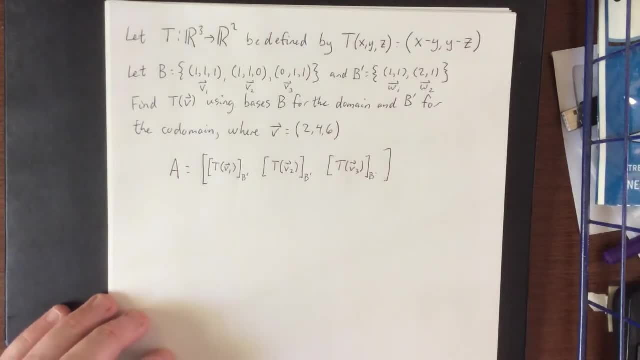 non-standard basis b prime. So let's go ahead and start by finding the image of all three of these vectors through our transformation. So image of v1 is going to be equal to t of 1, 1, 1, and again this image is supposed to be the. 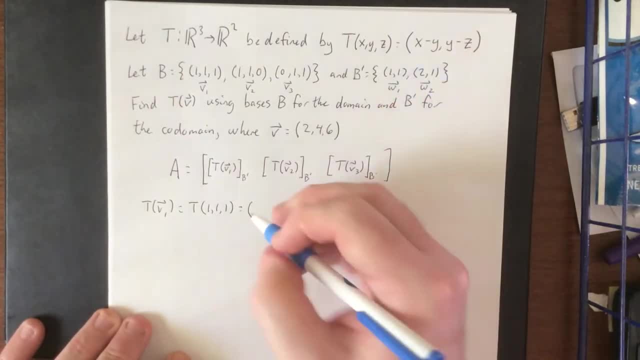 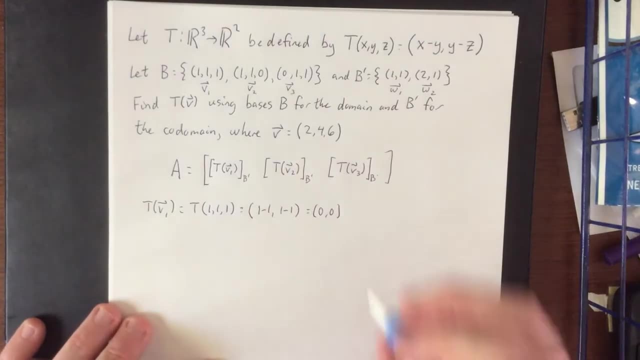 difference of the first two components and the difference of the second two components, So 1 minus 1 and 1 minus 1.. Thankfully we get the zero vector, which I can set up really easy as a linear combination of these two basis vectors by saying it's 0 times 1, 1 plus 0 times. 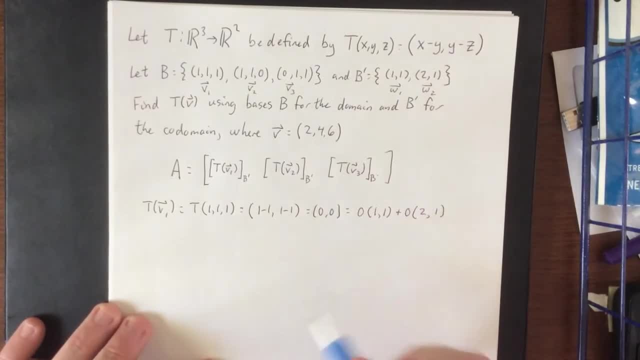 2: 1.. As such, the first column is going to wind up being 0: 0.. So the coordinate matrix of the image of v1 relative to basis b prime is going to be 0: 0 because of these two coordinates right here. 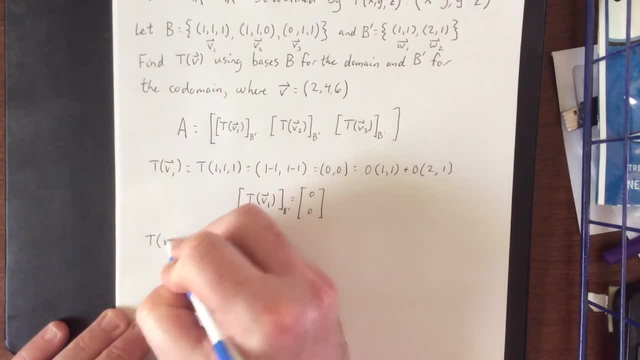 Let's do the same thing for the next one. t of v2 is going to be equal to t of 1, 1, 0, which again is going to be 0: 0.. So the first column is going to be 0: 0, and the next one is going to be 0: 0. 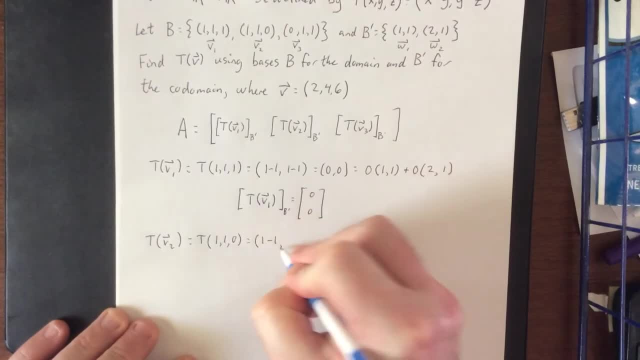 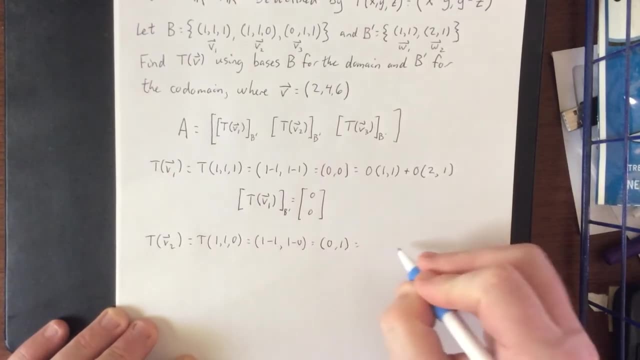 What we do is we take the difference of the first two components- 1 minus 1, and the difference of the second two components- 1 minus 0. What we wind up getting is 0, 1, which we are supposed to represent as a linear combination of the vectors 1, 1 and 2, 1.. So the thing that I'd 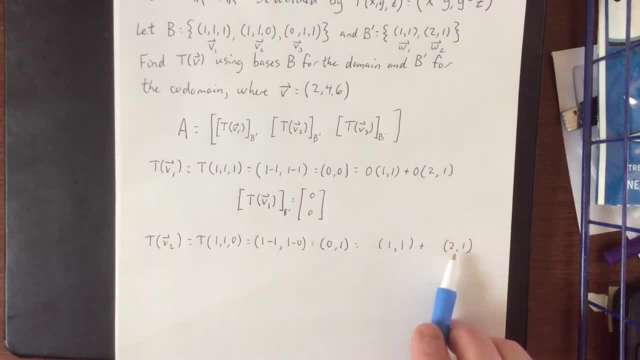 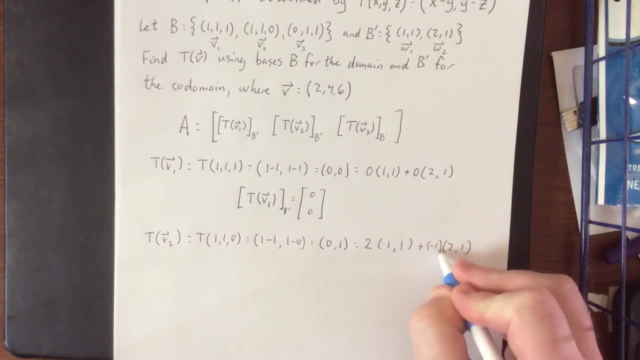 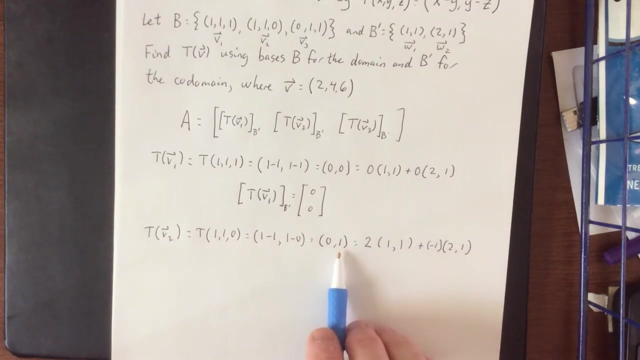 like to point out is that if I double the first vector and then subtract the second vector, we'll wind up with 0 and 1.. So double the first vector and then subtract the second vector. If needed, of course, you could set up c1 times 1, 1 plus c2 times 2- 1 is equal to 0, 1- and solve that. 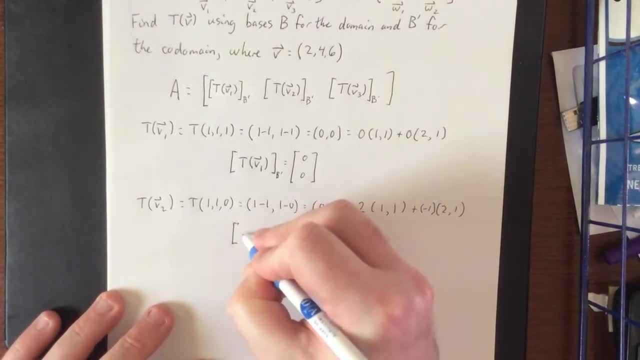 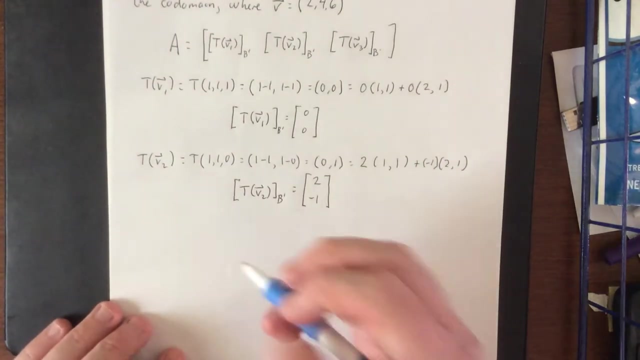 using a system of equations and a matrix. So the image of v2 relative to b prime is equal to these two coordinates: 2, negative 1.. We'll do the same thing for the last vector, That'll be t of v3.. 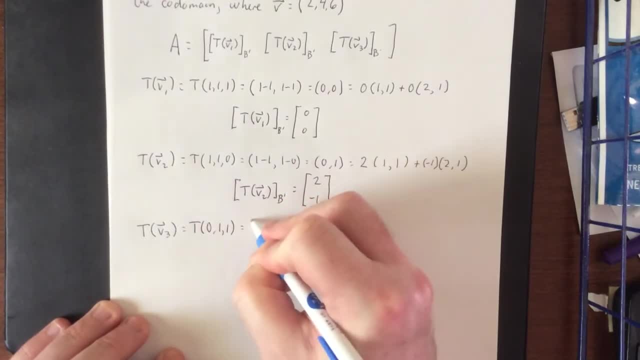 Our third basis vector. so 0, 1, 1, that is going to be equal to 0 minus 1 for the first component and 1 minus 1 for the second component. That'll be negative 1, 0.. And again we're supposed. 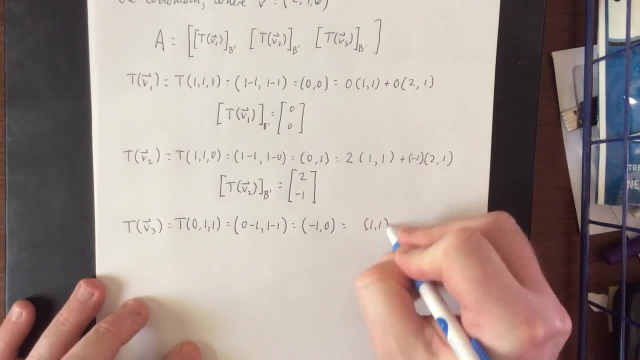 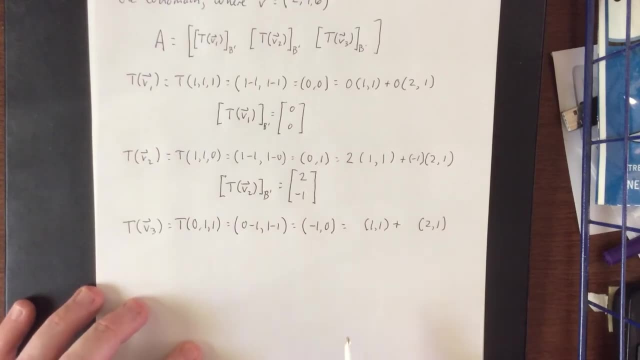 to be representing this as a linear combination of the basis vectors 1, 1 and 2, 1.. So I'd like to point out the same thing, as no, I guess it's not the same thing as what we did. If I take the first vector and subtract the second component, we'll get 0, 1 and 2, 1.. So that's. 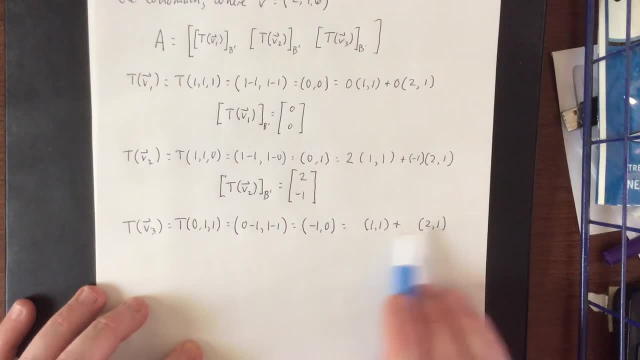 the second vector, The two components will be 1 minus 2 and 1 minus 1, which is exactly what we're looking for here. So the coordinates I'm looking for would be 1 of these and negative 1 of these. As such, the image of vector v3 relative to basis b, prime is the column matrix or coordinate. 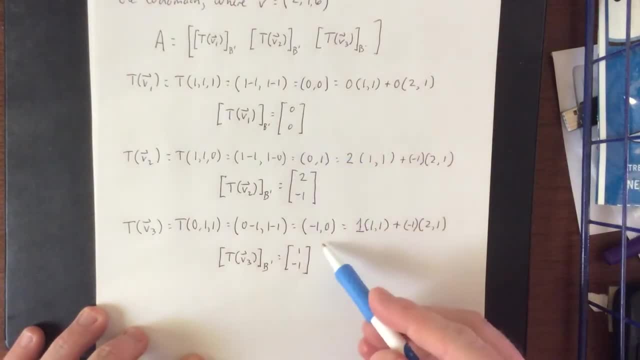 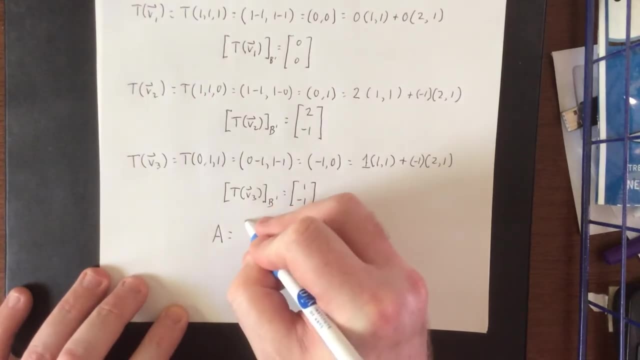 matrix 1 negative 1.. So these three columns will help us construct our matrix A relative to these non-standard bases. So this is going to be: A is equal to the 2 by 3, first column is 0- 0,. second column is 2 negative 1,. 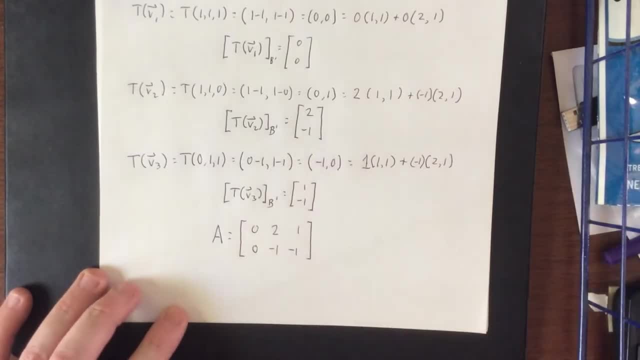 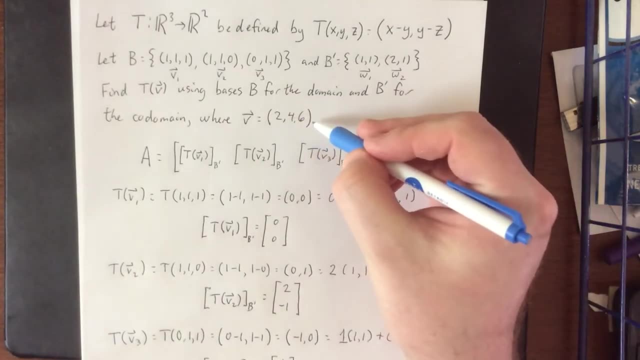 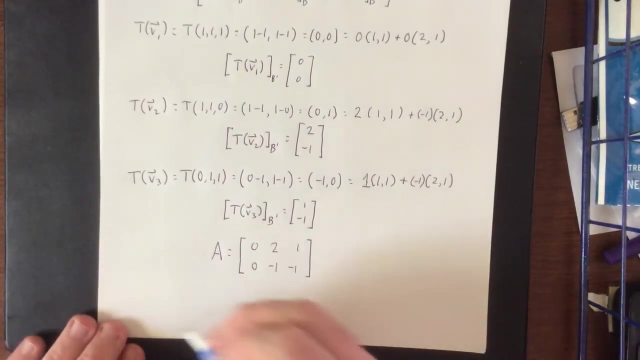 and the third column is 1 negative 1.. Now that we have this matrix, we will need to represent our vector v- 2, 4, 6, as a linear combination of these three basis vectors. So what we'll point out for 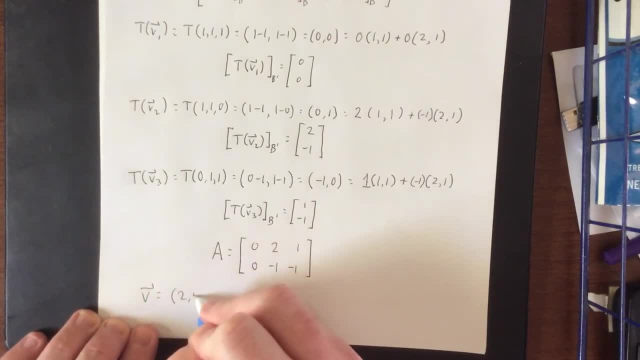 vector v is that v is equal to the vector v- 2, 4, 6, and the vector v is equal to the vector v 2, 4, 6.. Now we're going to set that up as a linear combination of 1: 1- 1, of 1 1- 0, and of 0: 1- 1.. 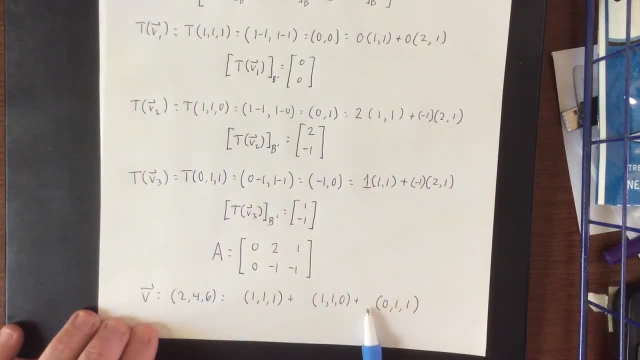 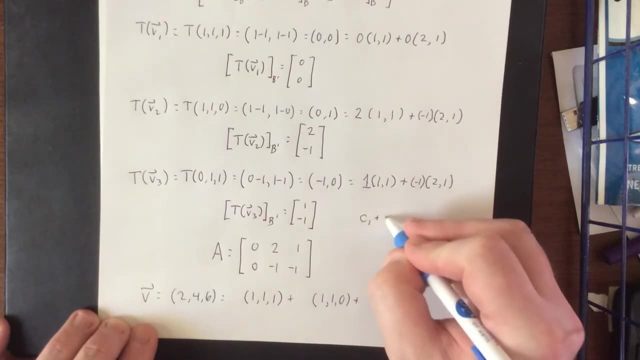 Now again, if you wanted to call these c1, c2, and c3,, set up a little system of equations. Actually, that's not a bad idea, Let's do that. So that's going to be c1 plus c2 plus 0 c3.. That'll. 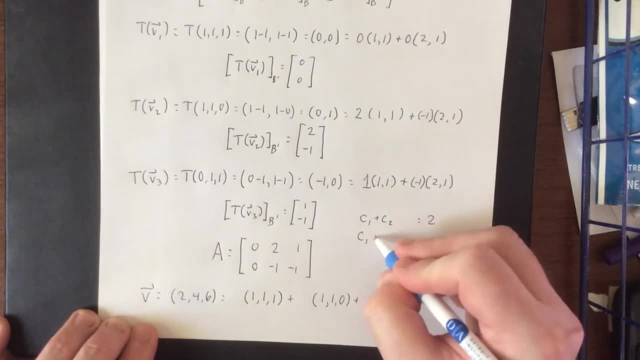 be equal to 2.. For the second component, that'll be c1 plus c2 plus c3, is equal to 4.. And then c1 plus no c2, and then c3. That's going to be equal to 6.. So if I take the second equation and I subtract, 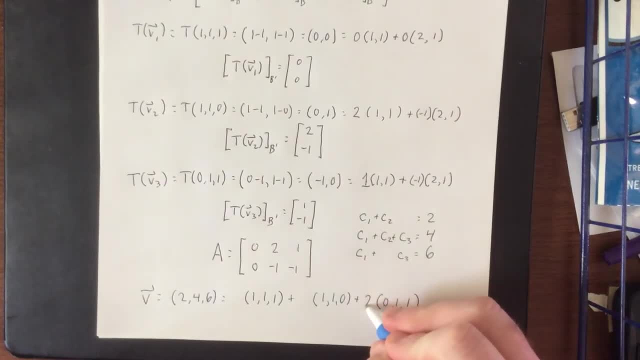 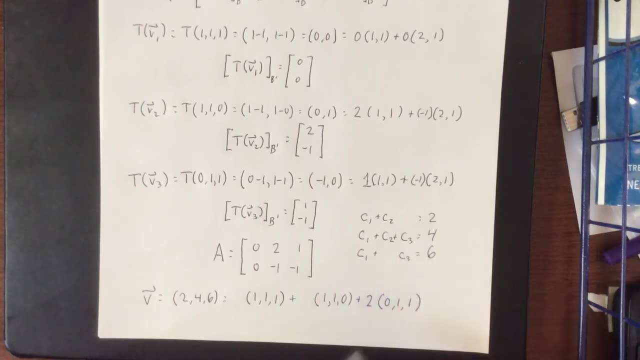 the first equation, we'll get c3 is equal to 2.. If I take the c3 equal to 2, or c3 equal to 1, or c2 equal to 0, 2 and plug it into the third equation, we'll get C1 is equal to 4.. If I take C1, 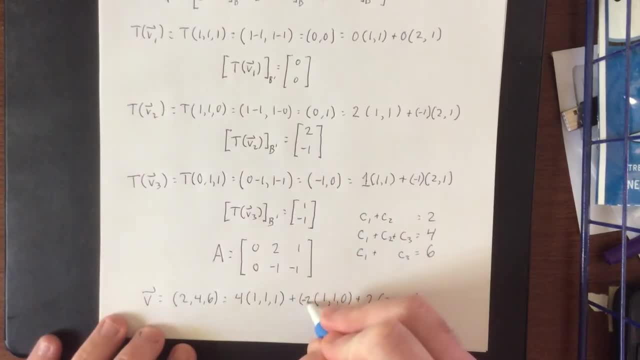 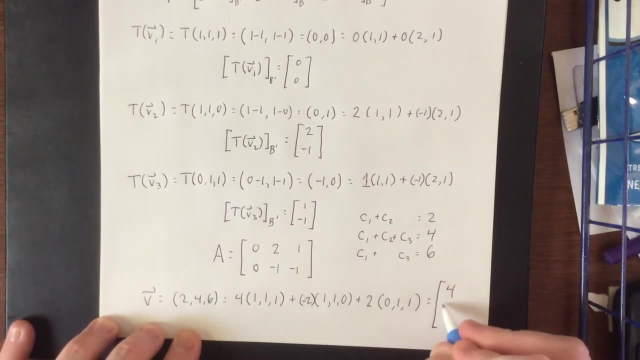 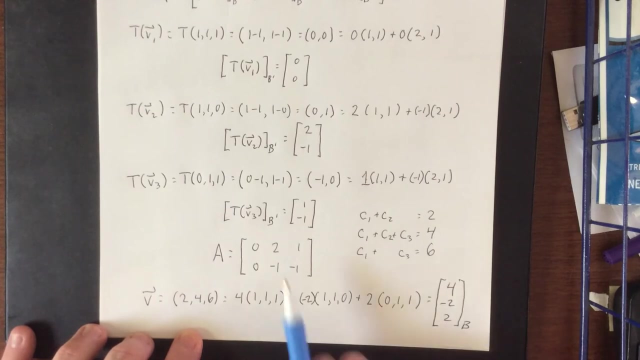 equals 4 and plug it into the first equation we'll get: C2 is equal to negative 2.. So that relative to the basis B means that we'll be dealing with 4 negative 2, 2 relative to the matrix B. So our next task is going to be to: 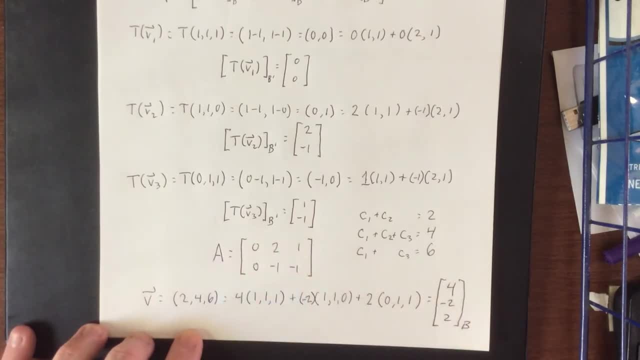 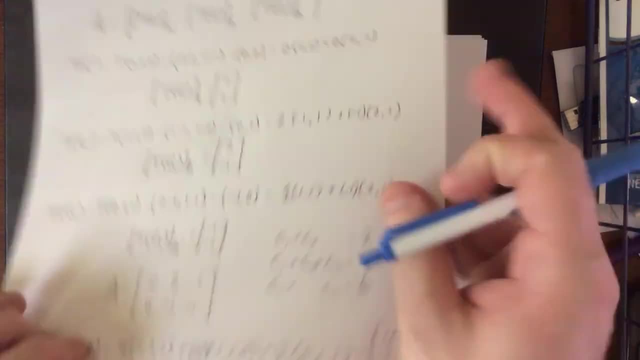 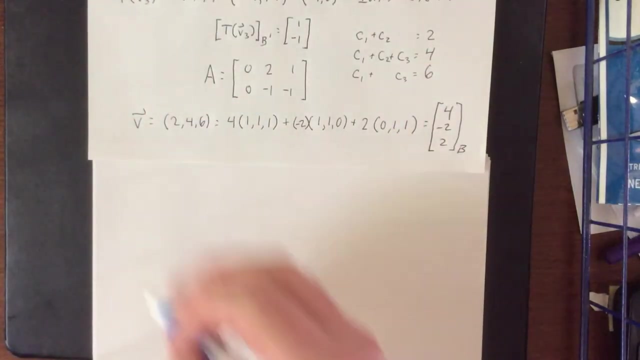 multiply A by this coordinate matrix and that'll give us the image relative to the basis B prime. Let's see if we can continue this on to a second sheet. There we go, There's physics working for us. So we'll say: next, We multiply. We'll be taking A times that coordinate matrix of 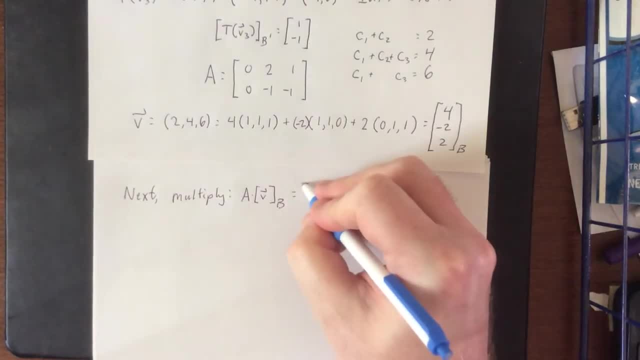 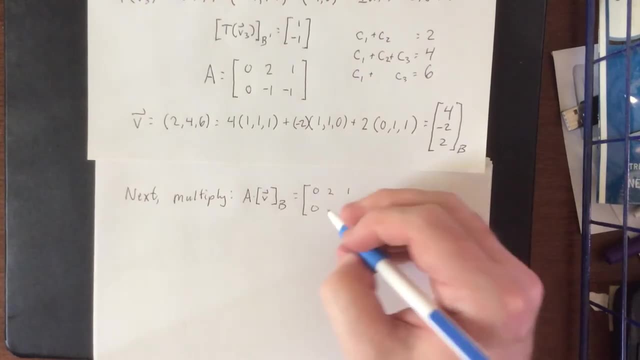 V relative to B. So that'll be the matrix: 0, 2, 2, 1, 0.. Hang on, I feel like something got. oh, nope, nope, we're good. Negative 1, negative 1.. We're going to multiply that by 4, negative 2, 2.. 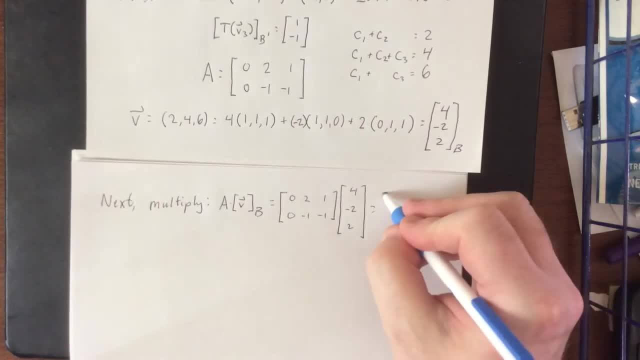 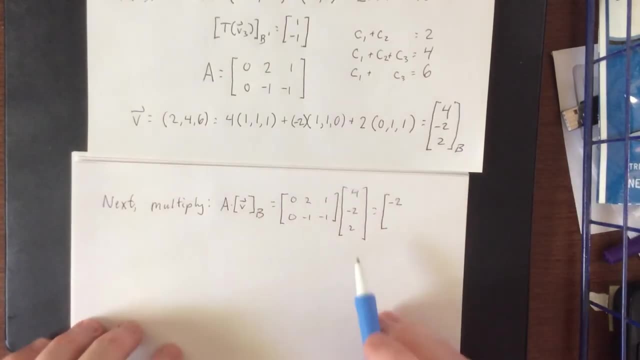 So a little bit of poking and prodding is going to be necessary. So 0 times 4,, 2 times negative 2, and 1 times 2.. That will give us negative 2.. and 0 times 4, negative, 1 times negative 2, and negative 1 times positive 2..